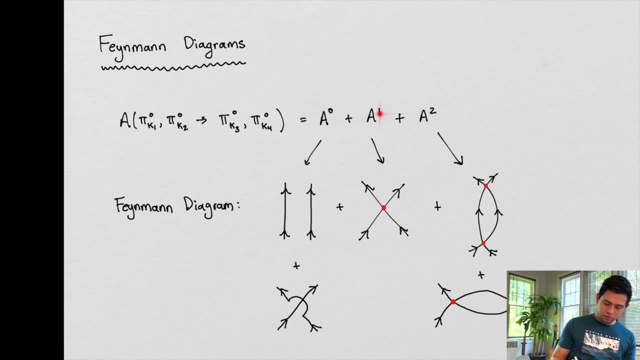 we had a zeroth order approximation. We said we had a first order. We're saying we have a second order And this approximation continues out n times, or an infinite number of times. And as we continue out an infinite number of times, we get high, we get more, higher degrees of. 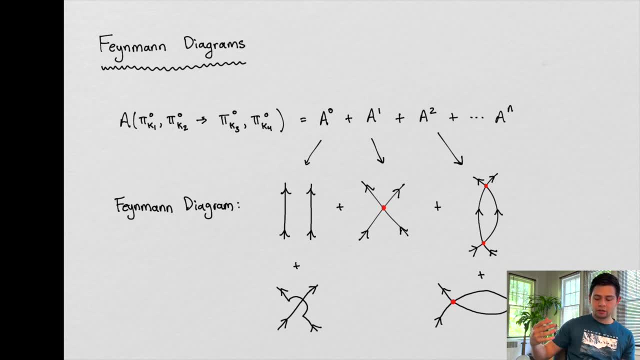 resolution, if you will, as to regarding how, how detailed we want to describe our scattering processes, And so what did Feynman do here? So so, so what we've been doing, so so, before I, before I go into Feynman, so what we've been, 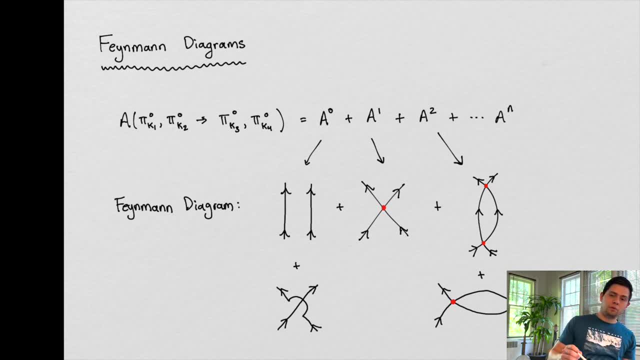 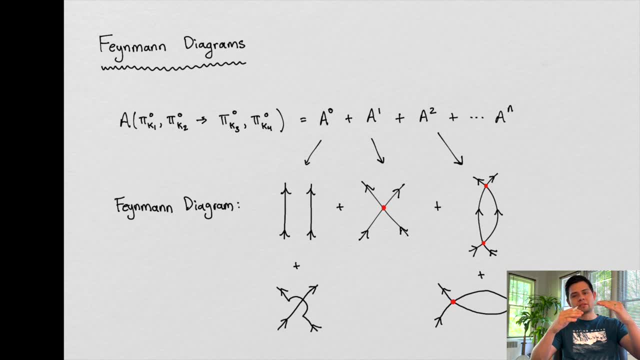 use wick, we've we, so we've. basically, we went from Wick's theorem: we use contractions, And then from the contractions we put them back. we, from the contractions, we put those back into our approximation form, right, And then from our approximation we derived a, a, the function that 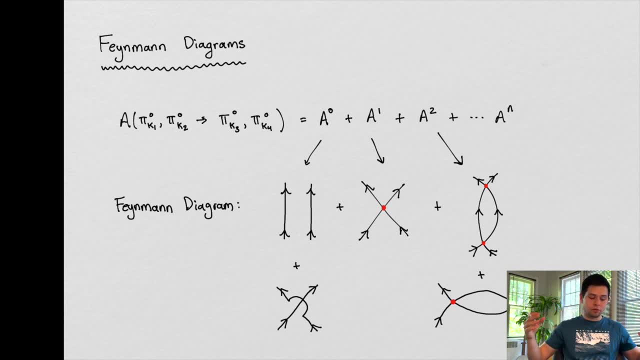 describes what was going on with that second degree term. Feynman's going to do here. Feynman is going to say: scratch all that, We're going to draw diagrams here. okay, We're going to draw diagrams so that we can make sense of what's going on, okay, So 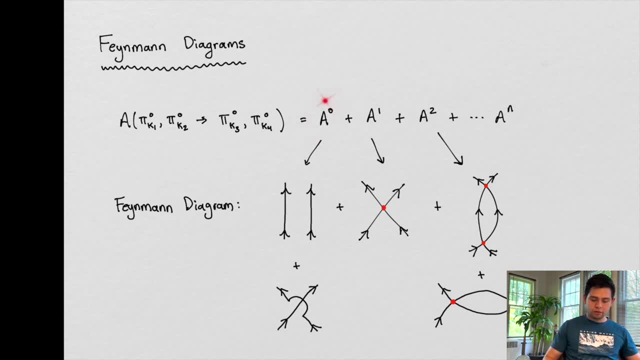 what do these diagrams look like? Well, this first order term is going to be a term that looks like this, where we have two incoming particles not interacting at all. okay, These two interacting particles not interacting at all are going to become two outgoing particles. 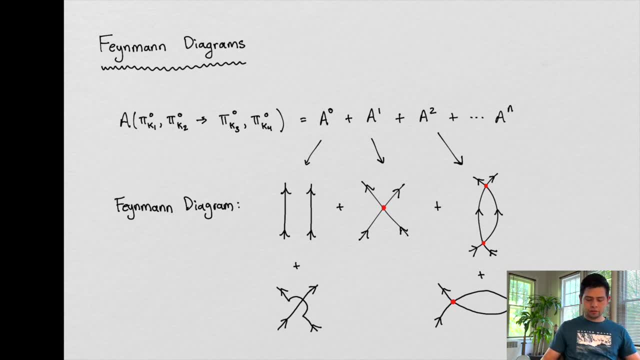 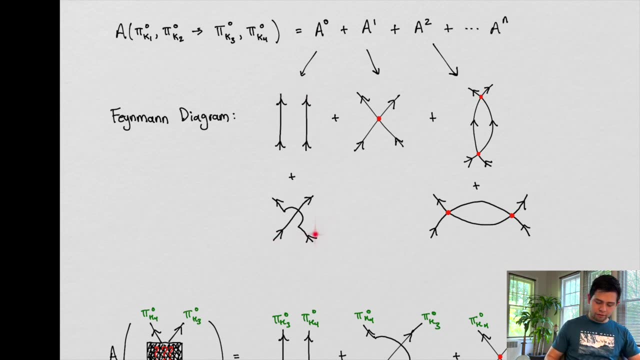 okay, There's no interaction at all between these two things. Another diagram in which something like this could happen is something like this: right, So we have incoming particle one and two and they end up at different locations in spacetime, right? If we can imagine these are. 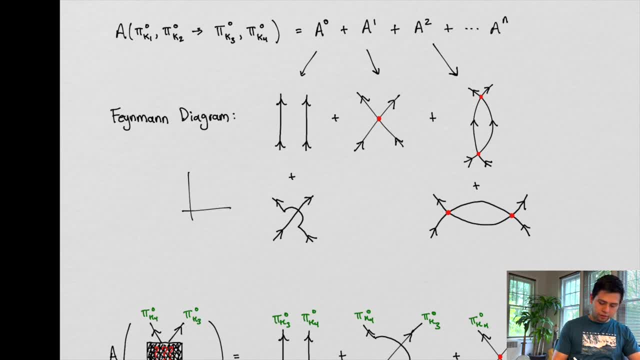 on a diagram of spacetime, right? So with time being here and space being here, they end up at different points in space, or at different different points of time, essentially, and space, But they've somehow crossed each other, but they didn't interact, right? So one way of thinking. 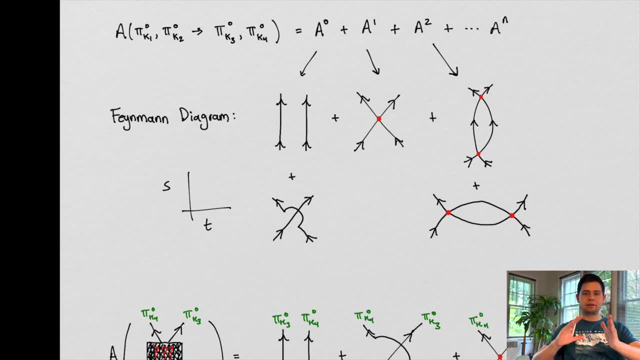 about, that is them being not within the same plane. say, right, So the two particles are not in the same plane, but so they're able to cross each other without interaction, right? They're able to cross each other without interacting with each other, right? So that's not too. 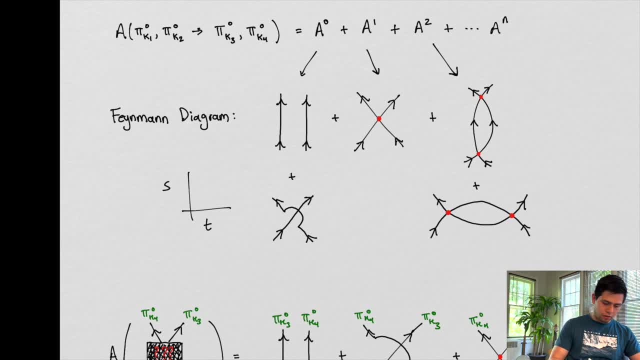 inconceivable To think about two particles ending up at two different spacetime points being, and so they're not interacting at all. right, So that? so this hump right here just depicts that non interaction, right? Okay, And then we have our first order term. So our first order term looks like this: 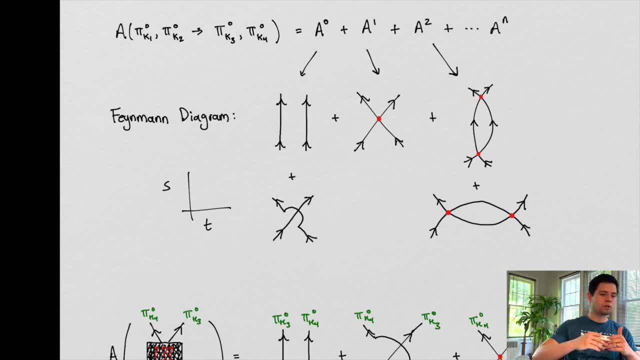 the order of the term right. So when we say first order, we have second order, zeroth order and so forth. zeroth order is where there's no, where there's no vertex right. So there's no point of, of of proximity between the two particles so that they 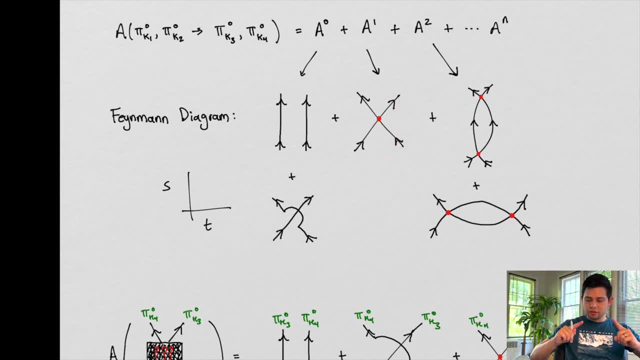 can interact. Here there is the, there is a vertex, So their paths do cross right. they do interact at a point. That's the first order term, So the order corresponds to how many vertices and that that's a key. 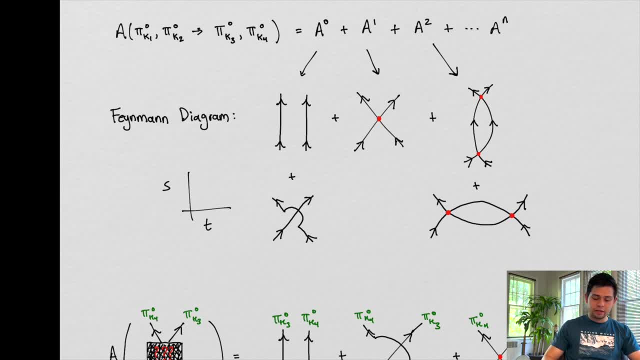 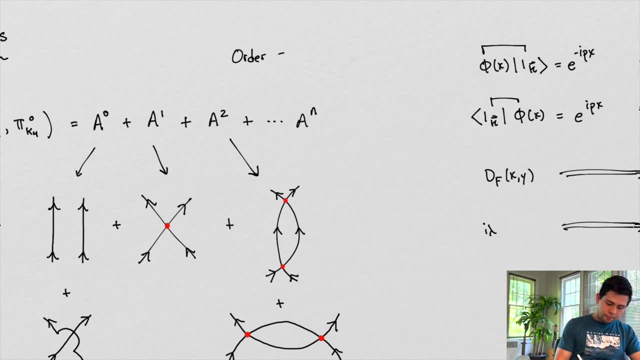 a key point here. The order corresponds to vertices And I'm actually going to write that down, All right, so order and vertices. Order, number of vertices. I don't know if I spelled vertices right, But this is a key point here. This right here is something to ingrain into your. 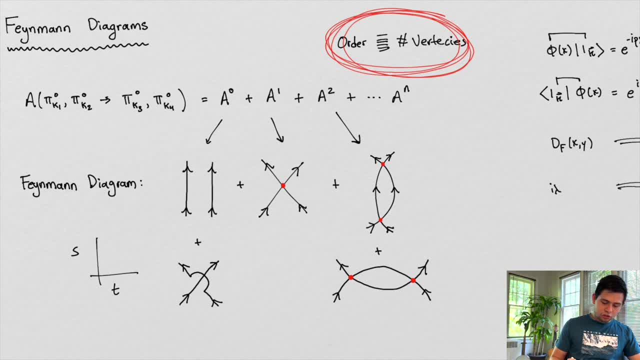 brains, Because each term here, each term here. so the first order term corresponds to all the terms or all the diagrams in which the particles could only interact once. Okay, the second order term corresponds to diagrams that might look like this, right? So these are diagrams that. 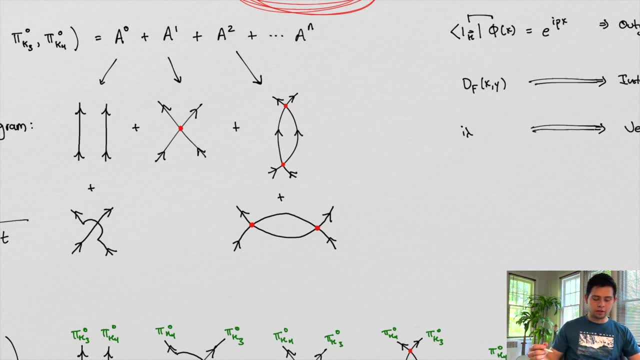 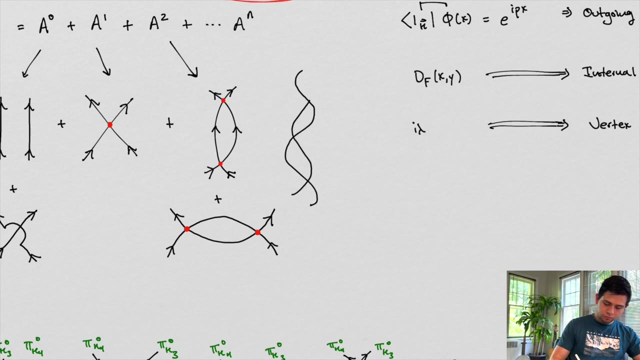 describe particles that interact twice. Okay, so interaction and then outgoing An nth order term. Okay, I'm going to try to draw an nth order term, Something that might look like this: All right, so what is this? We have an interaction here. 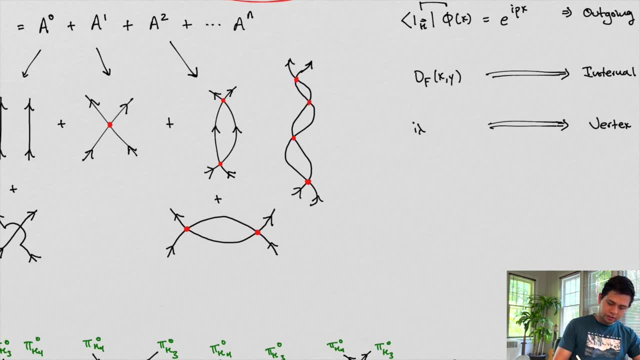 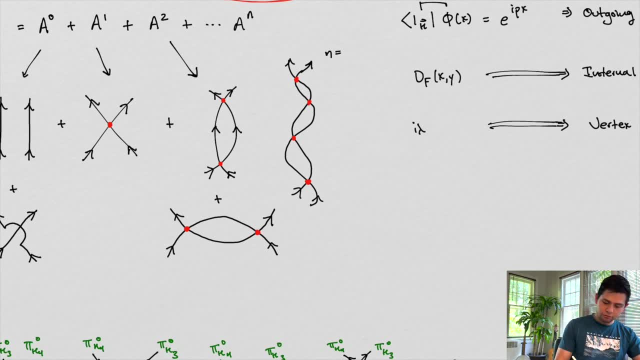 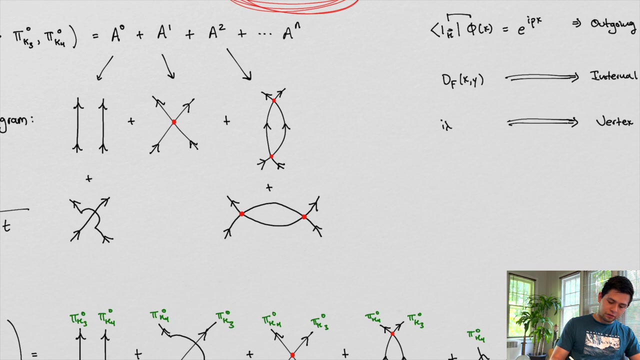 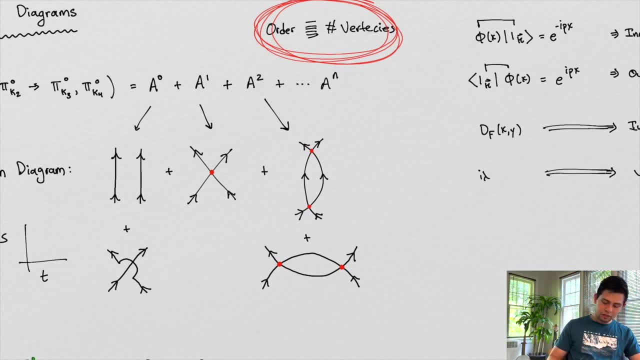 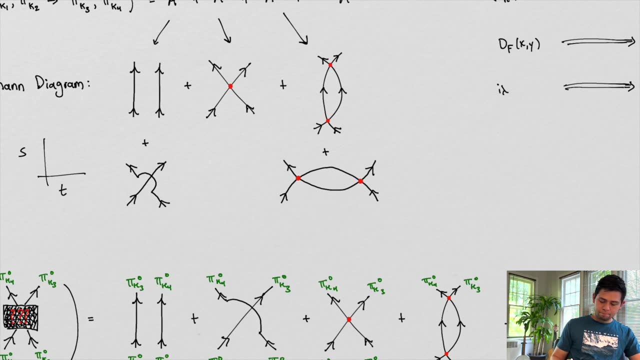 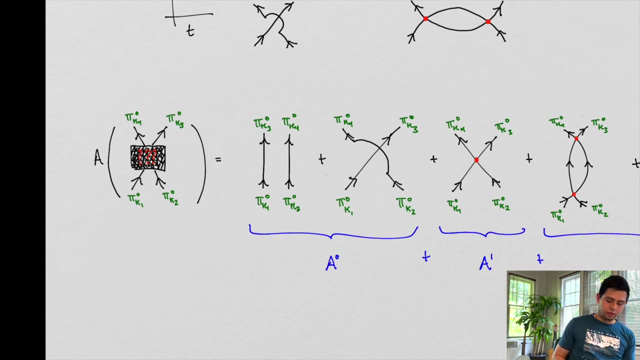 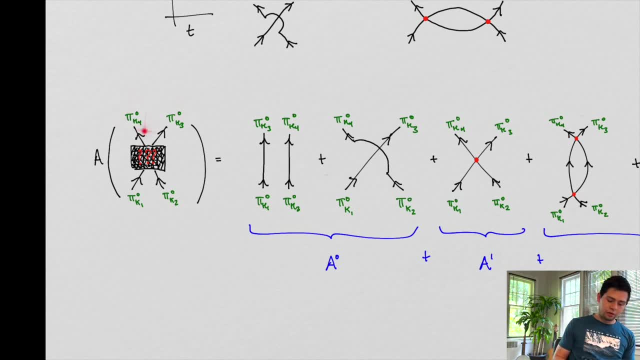 any assumptions at this point. and then we have two outgoing particles. okay, so we're going to approximate what we want to. we want to approximate this amplitude and two. the way we approximate this amplitude is by saying we add up all the zeroth order terms, so that'd be these two terms. then we 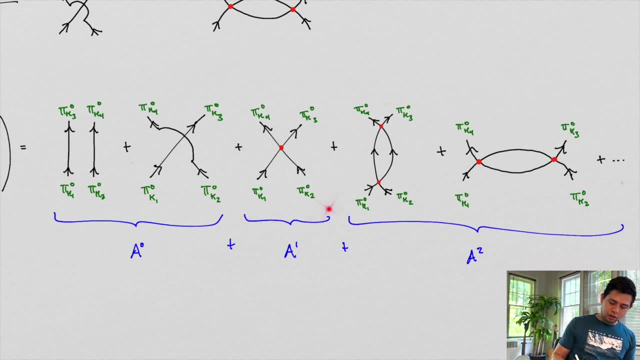 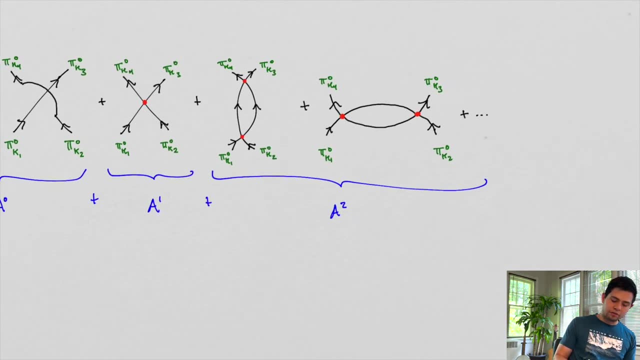 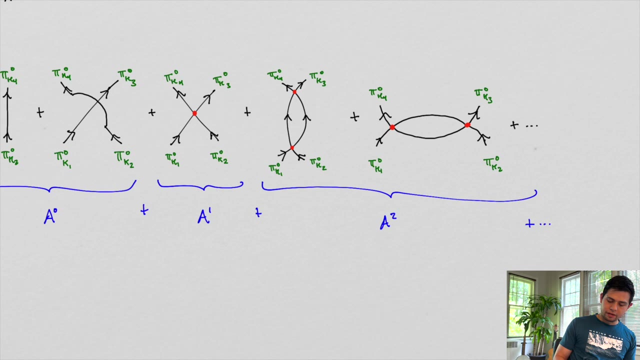 add up all the possible- uh, all of the possible- first order terms. so this is the point of only one interaction. and then we add up all of the second order terms and so forth. okay, how is this actually helping us for calculations? all right, so you might ask that 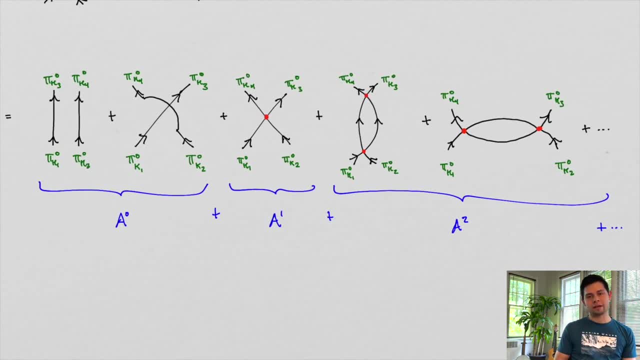 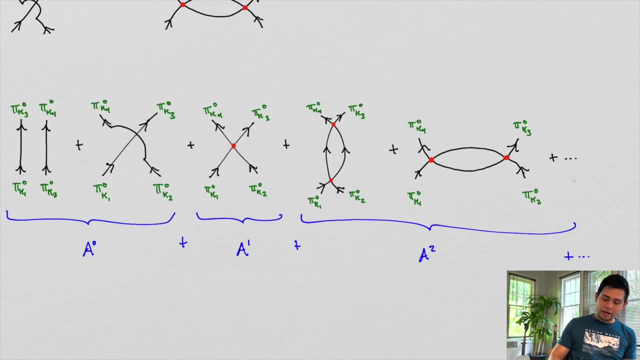 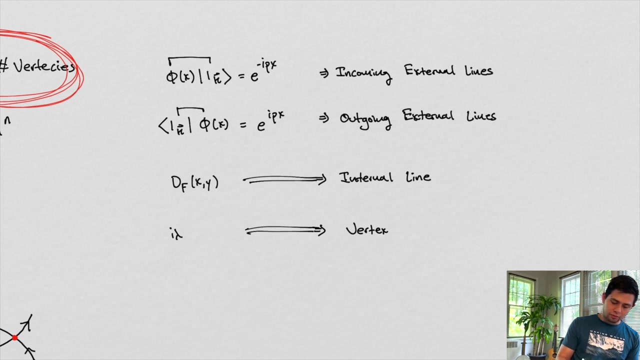 question: how exactly is that, this diagrammatic way of thinking about amplitude calculation? how is this helping us? well, the way it's going to help us is: we're going to look, we're going to come here now and i want to move this down a little bit. these are what are called the feinman rules. 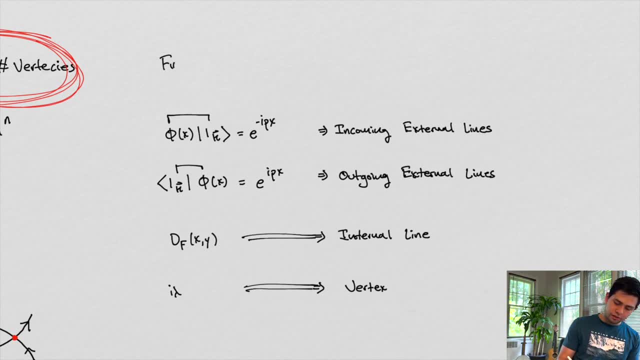 if feinman rules specifically for the, the three of five and four, and these are those four rules called byokes, and we like them in the shaded order, and this is the spokenρά code. so this is the bound constant for the, the five- four model or the fourth power model. right, we're going to find out, though, that the 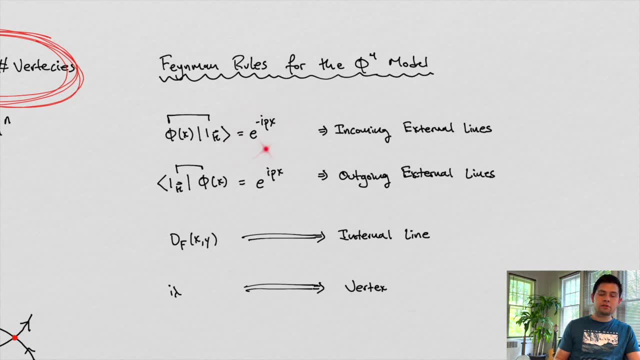 rules are really not that different for more generalized models. okay, and we'll. we'll see that later on. but we're going to say, okay, we had all those contractions right in our calculations. important contraction that we've seen before. This contraction is going to be associated with. 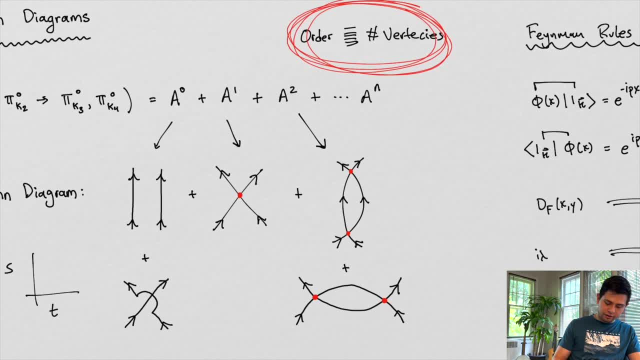 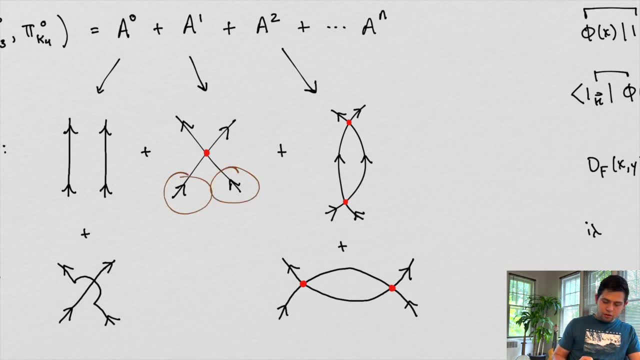 incoming external lines. So let's look at a diagram again. Let's take a look at this diagram right here. So these two guys right here are going to be given this factor of e to the ikx and e to the ikx minus ikx, right? So these are two particles that have momentum k. 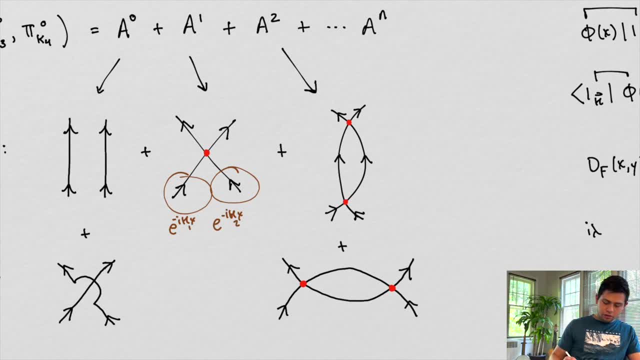 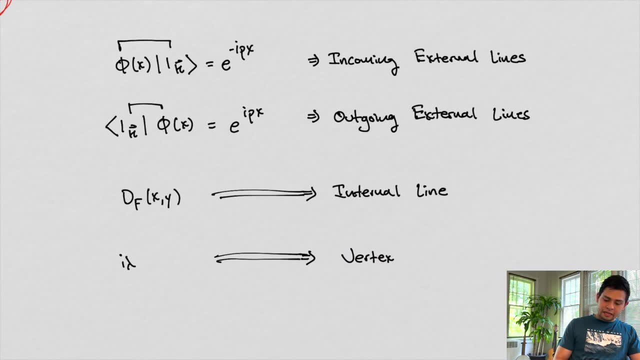 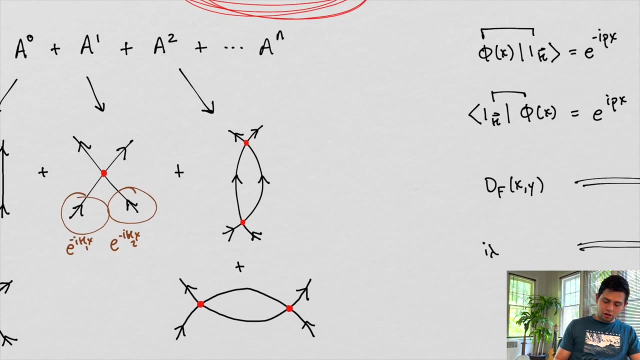 so say k1 and k2, and they're going to be given this exponential term. okay, That's the incoming external lines. The outgoing external lines, they're just going to have an opposite sign on the exponent. So, the outgoing external lines, they're just going to have an opposite sign on the exponent. So 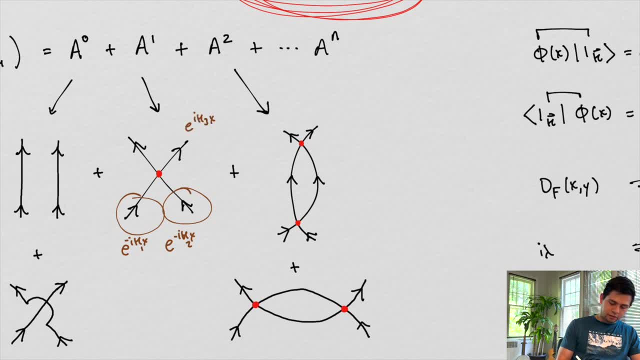 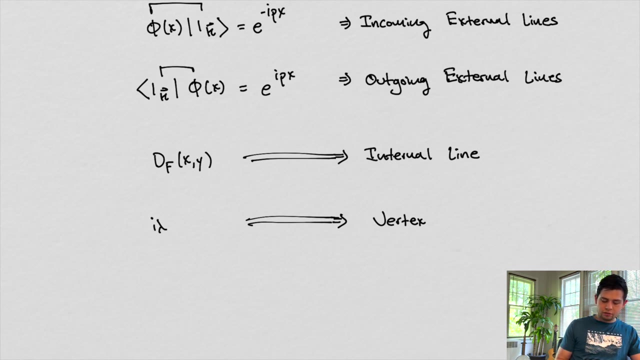 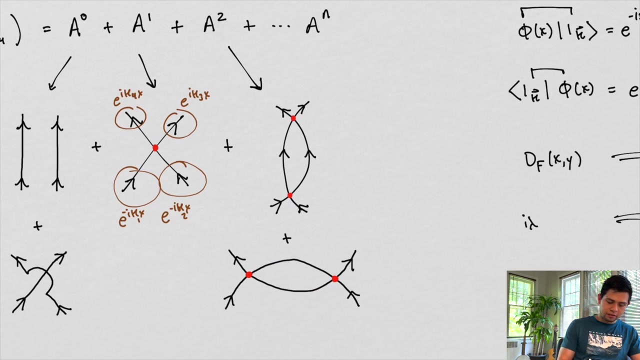 e to the ik3x and e to the ik4x. That's these guys right here, okay, And then. okay, so this one. so internal lines. so this is the Feynman propagator. Now, we don't have an internal line in this diagram, but in this diagram here. 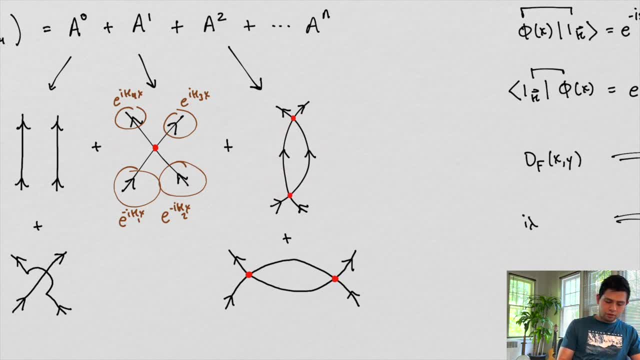 but we do have internal lines here, right? So this is an internal line and this is an internal line, and this is an internal line and this internal line here and this internal line here, these are going to be given d, f, k, y, right? So this is not k, x, this is x. 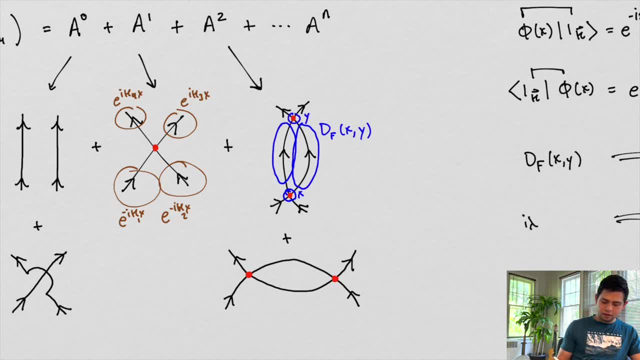 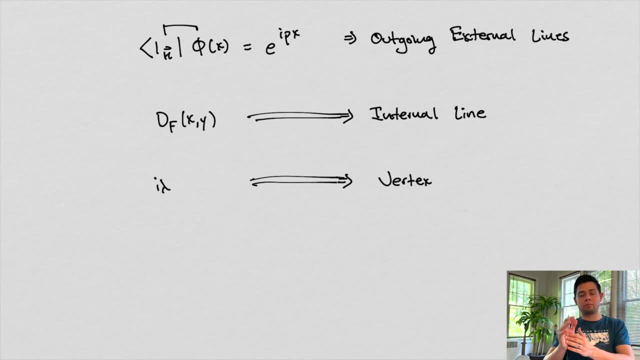 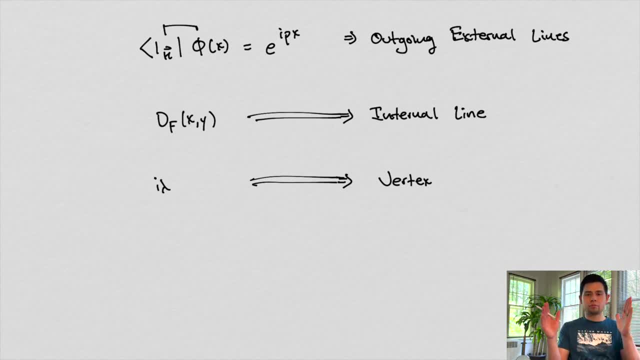 in two points at space-time and they compare the two points or they calculate what the amplitude is going to be to for a particle to travel between this point and the next point, and the further the points are from each other, that amplitude decreases exponentially. 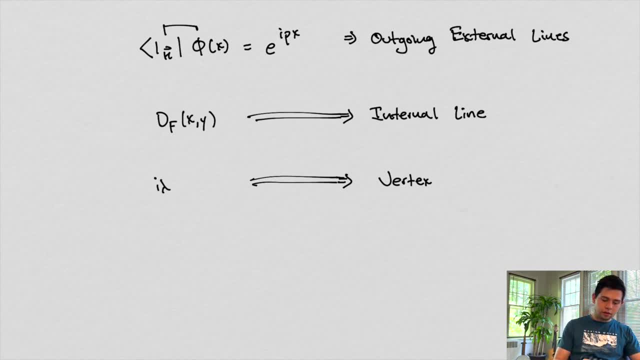 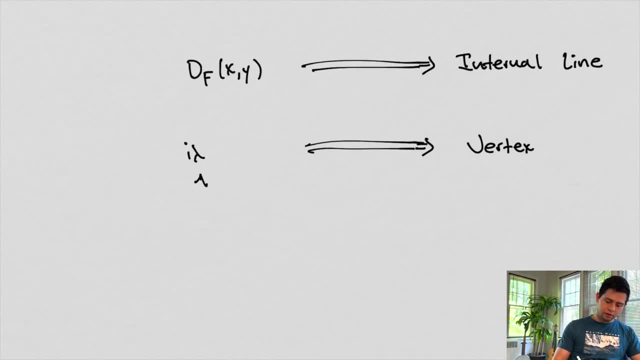 for very important reason, This guy right here is going to be a very important thing we want to talk about when we're talking, when we start talking about renormalization, stuff like this, This couple, this is a coupling constant. essentially, This is a constant that's going to tell us 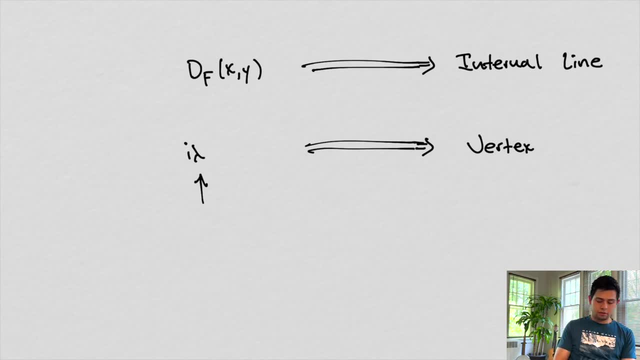 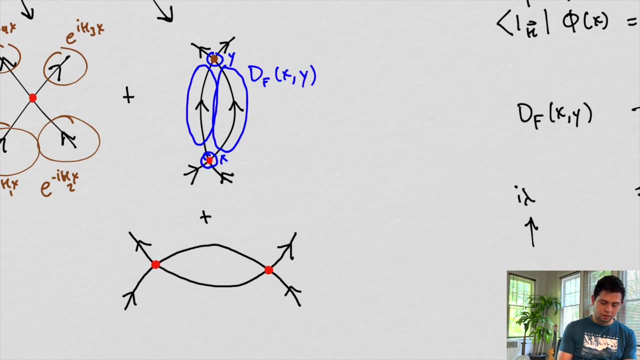 something about here. we'll we'll go to the diagram here. So it's going to tell us something about what's going on between the degree of coupling- here I'll do that in a different color- the degree of coupling between the two particles that interact with each other at that point.